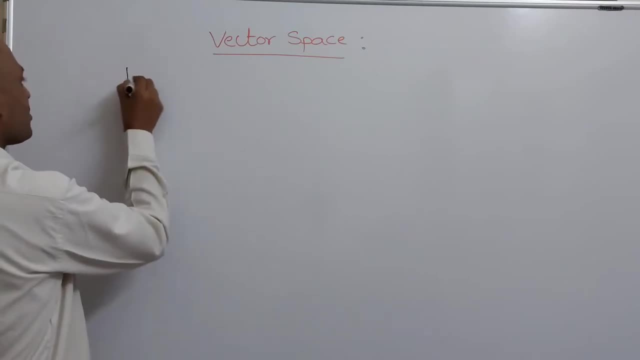 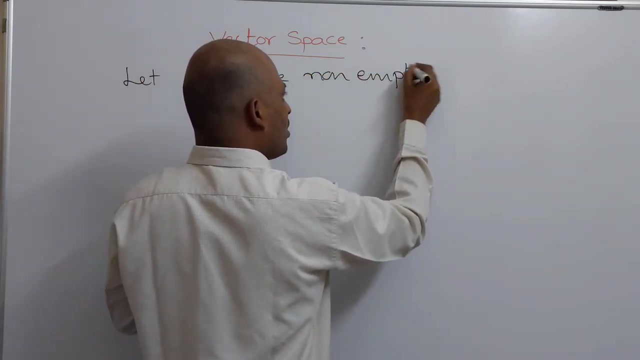 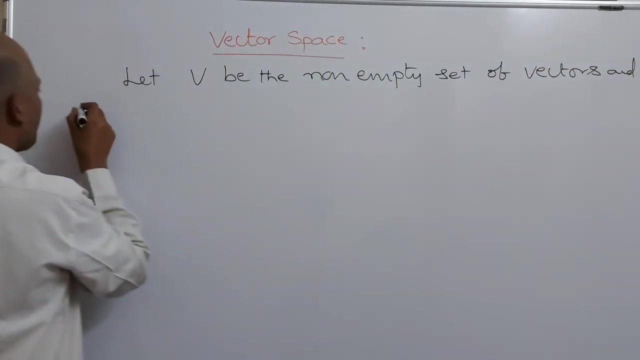 Let capital V be the non-empty set of vectors. Let capital V be the non-empty. let capital V be the non-empty set of vectors. non-empty set of vectors. and capital F be the. capital F be the field of scalars, capital F be the. 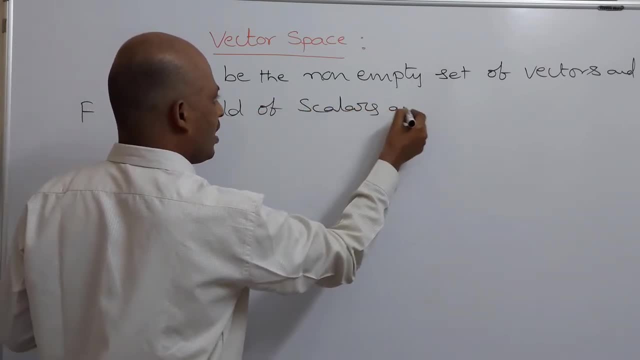 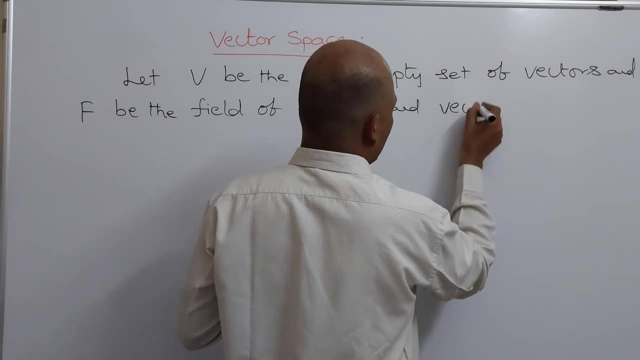 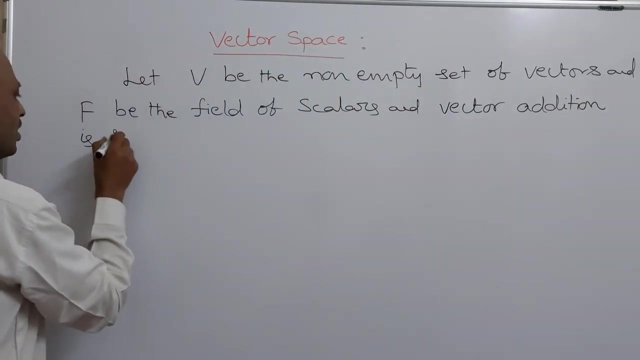 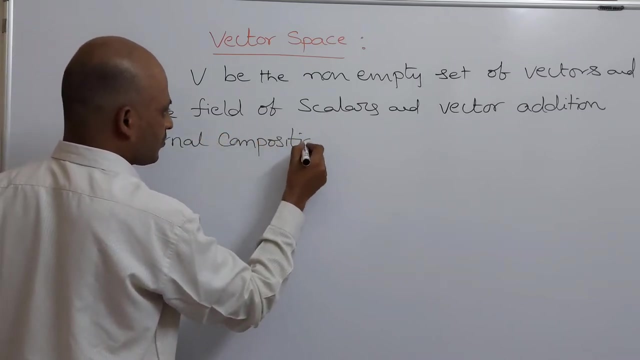 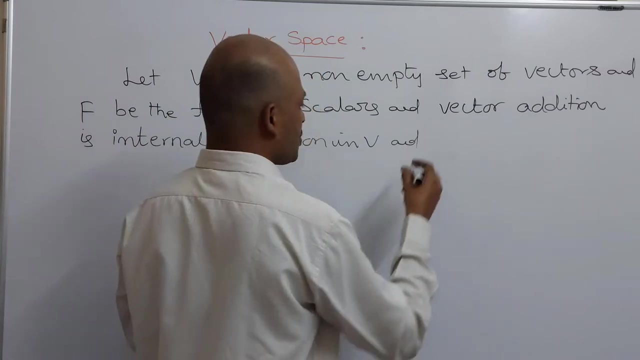 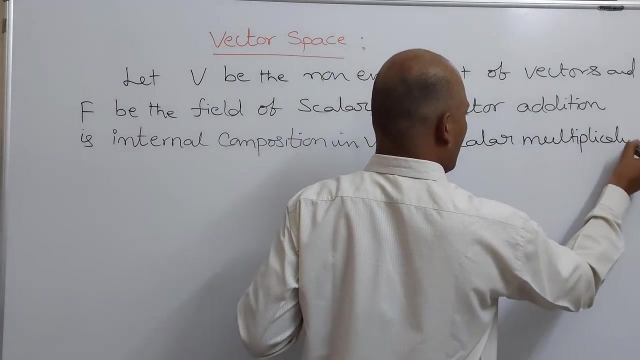 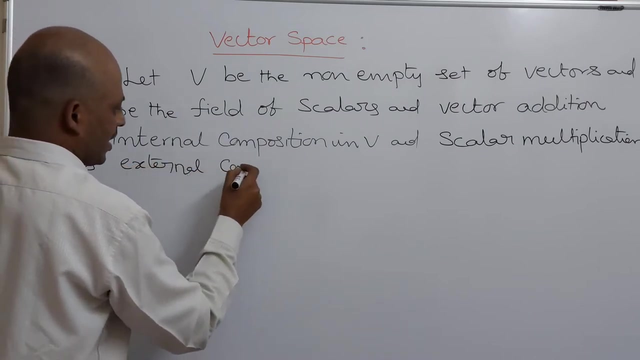 field of scalars, And vector addition is internal composition. inverse Vector addition is internal composition. Vector addition is internal composition in capital V and scalar multiplication is external composition in V. Scalar multiplication, Scalar multiplication, Scalar multiplication is external composition. external composition in capital V over capital F. 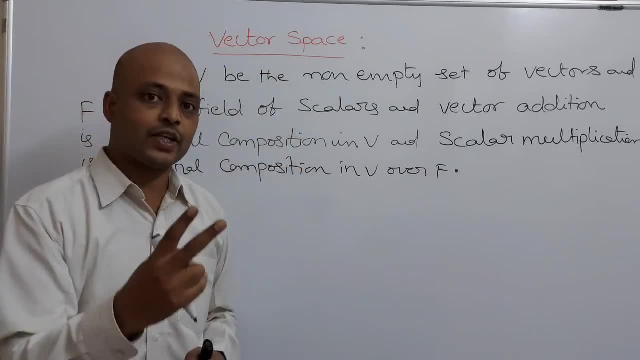 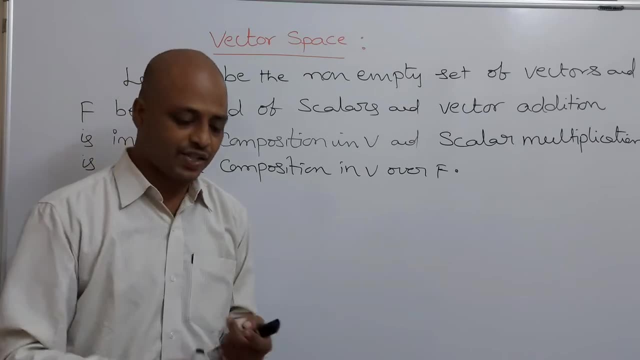 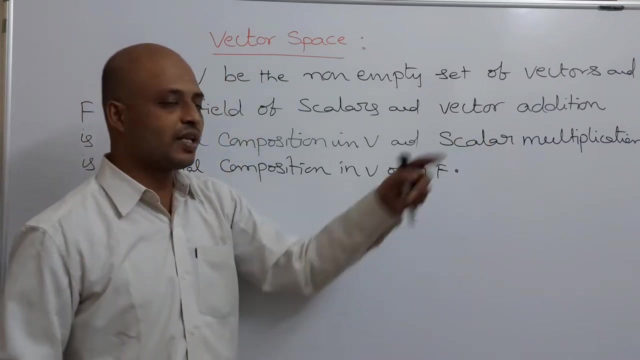 Observe that To define Vector Space we take two sets: V is the non-empty set of vectors, F is the field of scalars And we take two operations: Vector addition as internal composition. Vector addition as internal composition. Scalar multiplication as external composition. 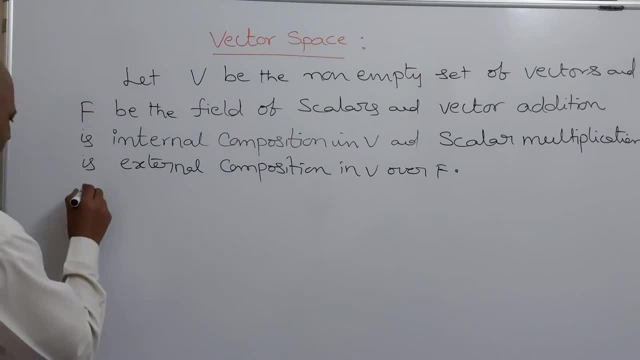 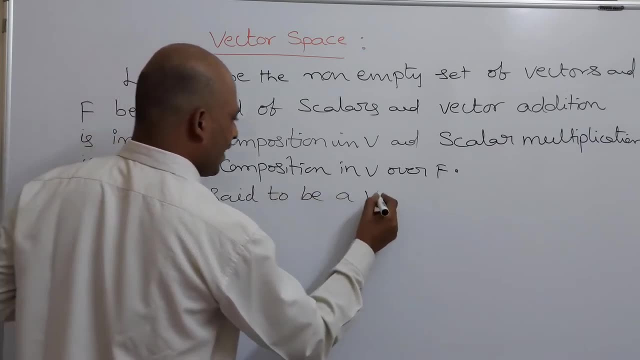 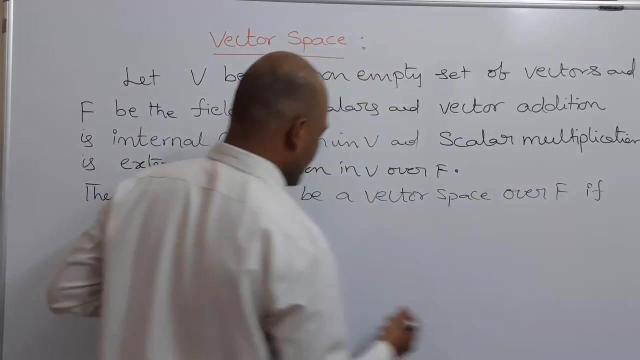 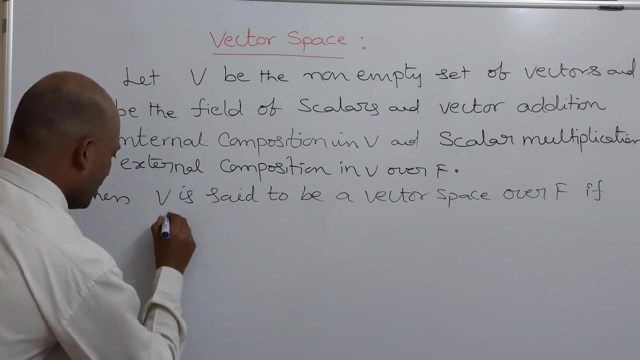 Scalar multiplication as external composition, Then capital V is said to be capital V is said to be a vector space, a vector space over capital F, if it satisfies the following two major conditions: If it satisfies the following two major conditions, The first one: 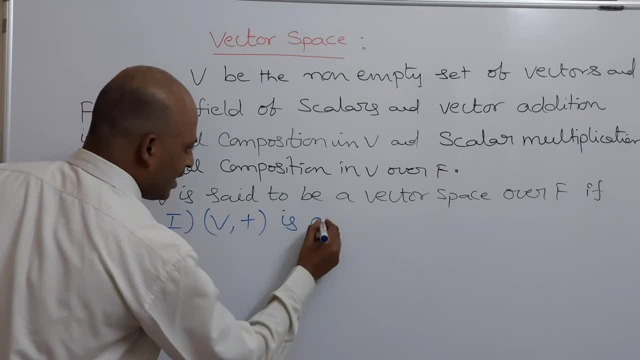 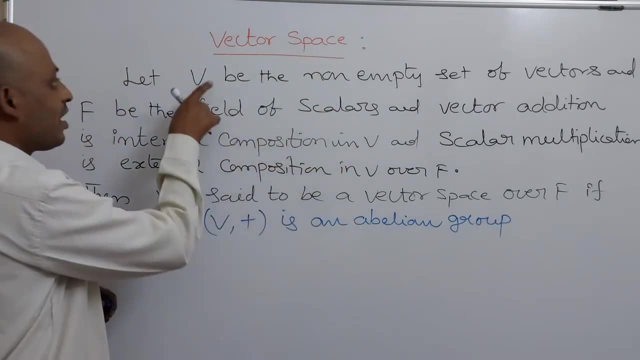 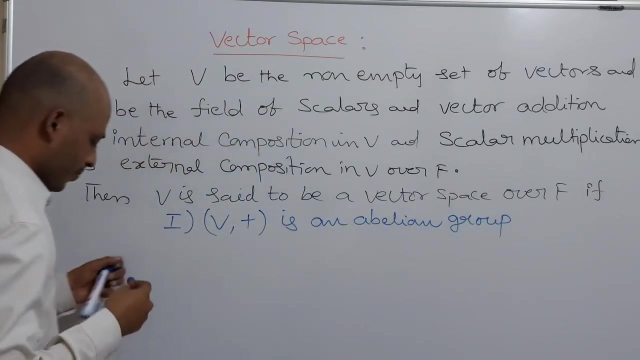 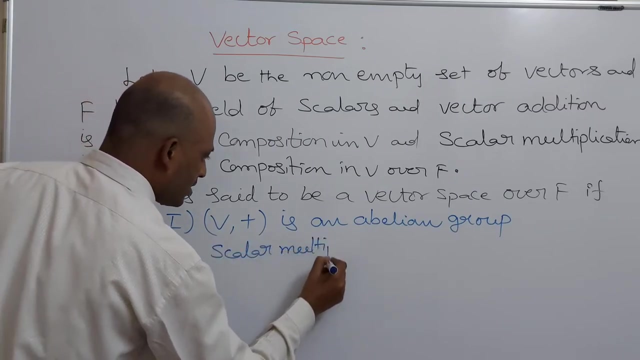 V with respect to plus. V with respect to minus Is a abilian group. V with respect to plus is a abilian group. The set of vectors V with respect to vector addition method is an abilian group. The second one, Scalar multiplication property. 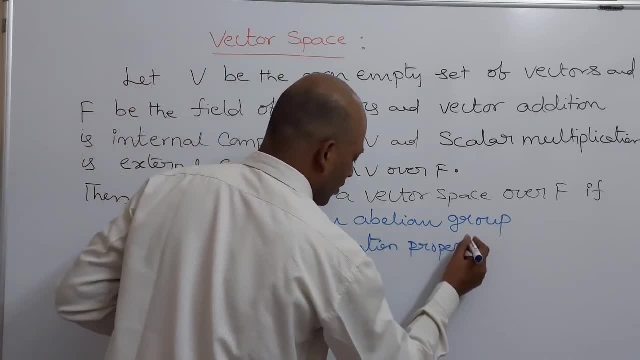 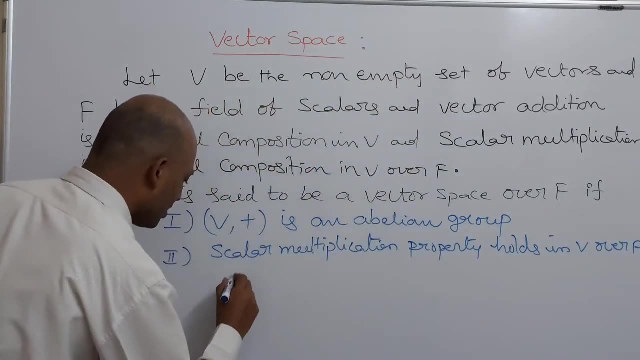 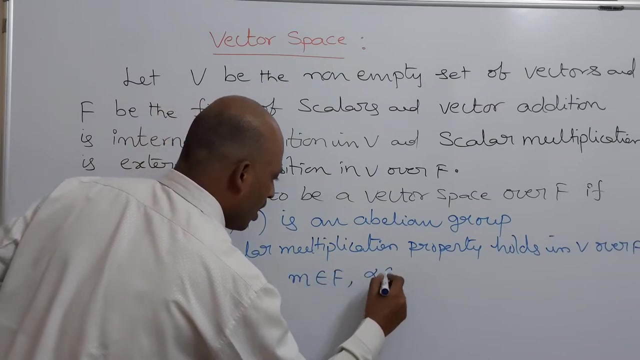 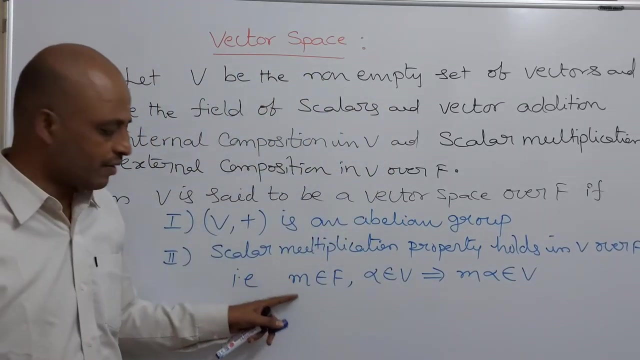 Scalar multiplication property: natural holds in V over capital F. What is scalar multiplication property? That is small. m belongs to F. alpha belongs to V implies m. alpha belongs to V. M belongs to F. alpha belongs to V implies m. alpha belongs to V. Observe that V with respect to 2 plus is an abelian group. 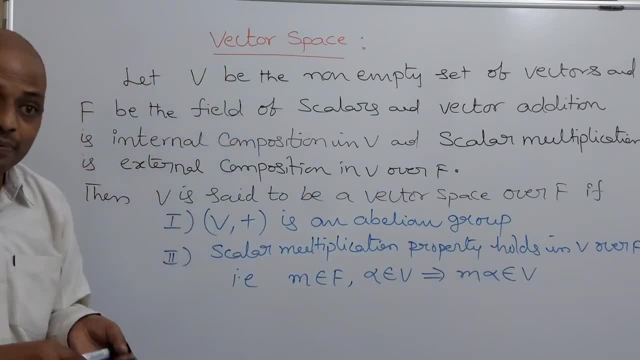 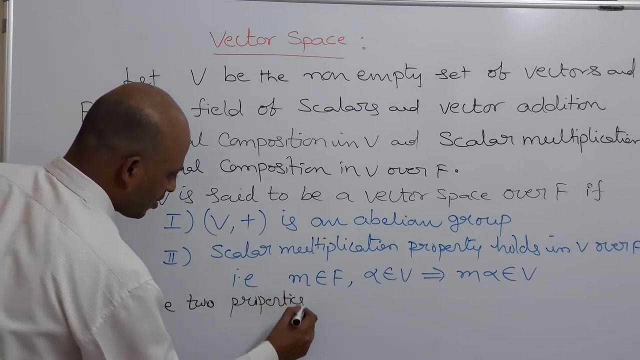 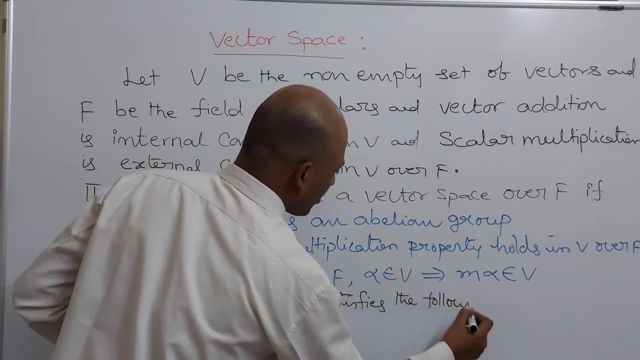 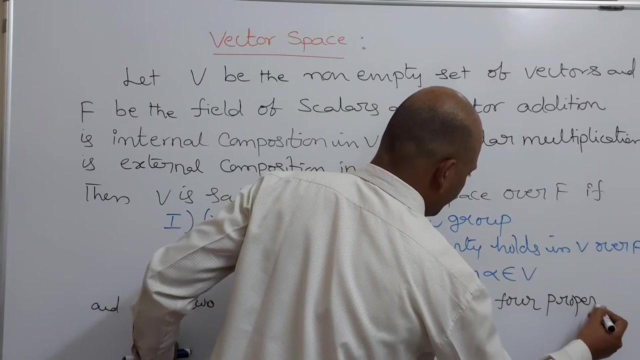 and scalar multiplication property holds in V over capital F, and these two are known as major conditions. And these two properties or these two conditions or properties satisfies. satisfies the following: the following four conditions or four properties, Okay, Or four axioms: The above two properties. satisfies the following four conditions: 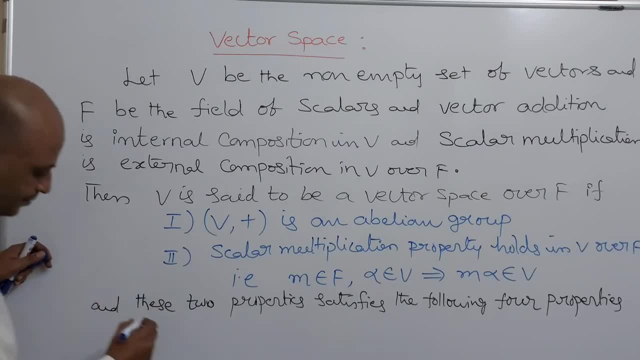 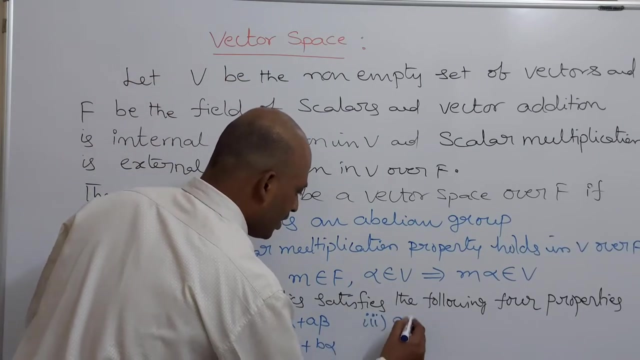 The first one is. the first one is: a into alpha plus beta is equals to a alpha plus a beta. And the second one is: and the second one is: a plus b into alpha is equals to a alpha plus b alpha. And the third one is a into b- alpha is equals to ab into alpha is equals to a alpha into b. 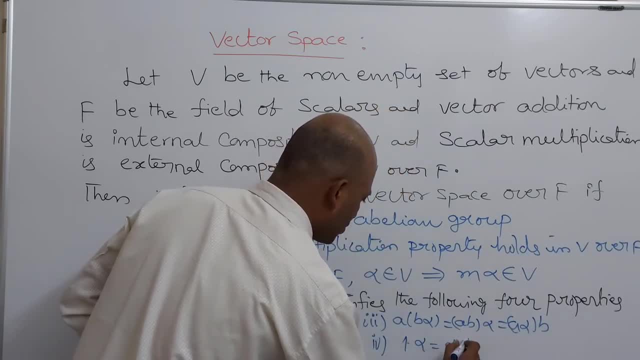 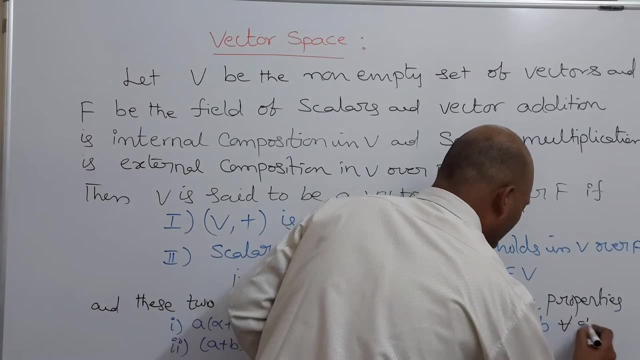 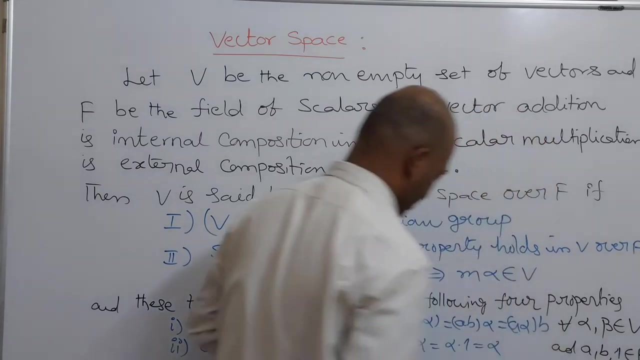 And the fourth one is: 1 into alpha is equals to alpha, into 1 is equals to alpha comma, where You observe that For all alpha comma, beta belongs to V and a comma, b comma 1 belongs to the field F, So any set capital F. 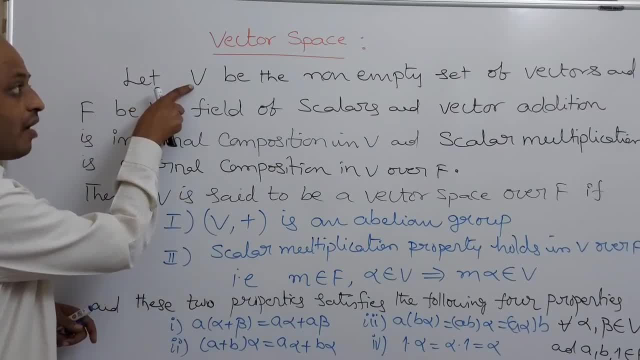 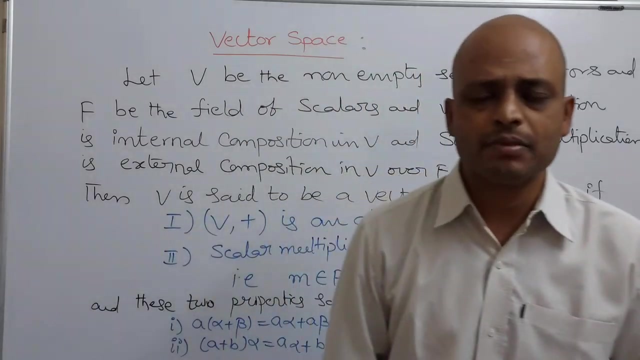 capital V over capital. any set capital V of vectors over capital F satisfying all these four properties is known as a vector space, is known as a vector space. I repeat again the definition, which is very, very important one, To prove every theorem, to prove every property. we need this definition. 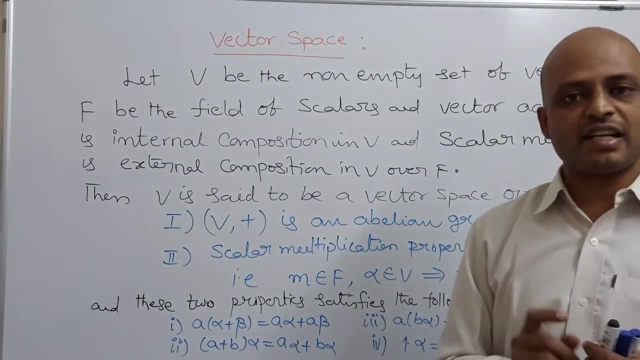 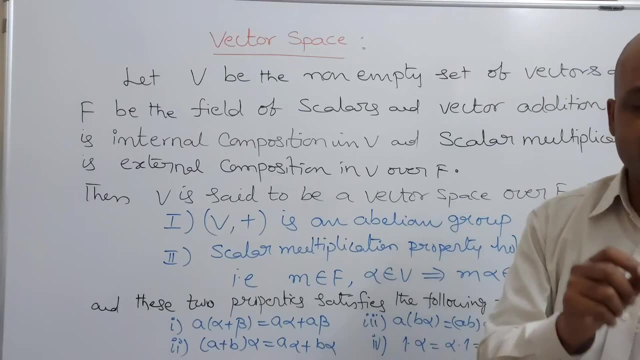 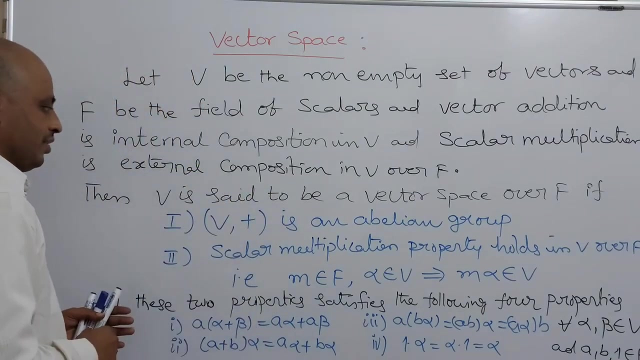 So learn the definition first carefully. Capital V is the non-empty set of vectors. Capital F is the field of scalars, Vector addition. vector addition is the internal composition and scalar multiplication is the external composition. in V over capital F, Then V is said to be a vector space over capital. 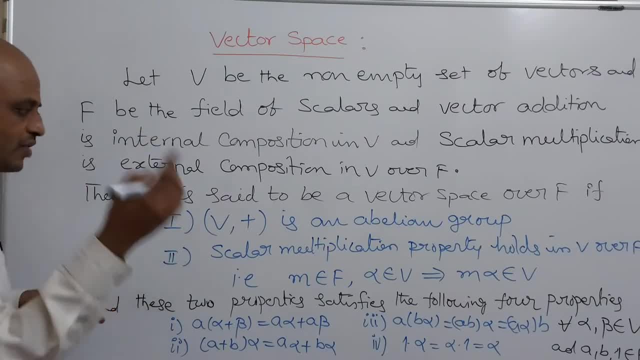 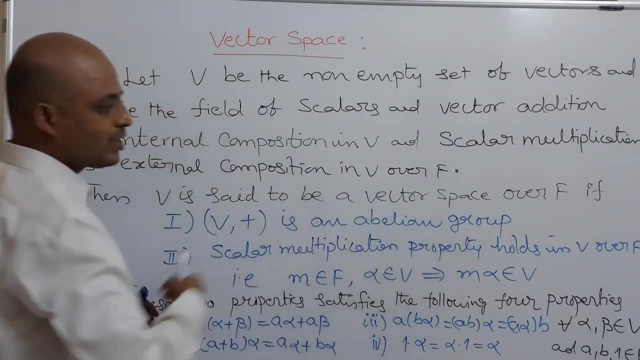 F if it satisfies the following two conditions. The first one, V with respect to 2 plus, is an abelian group. The second one, scalar multiplication property holds in V over capital F. That is, m belongs to F, alpha belongs to V implies m alpha belongs to V. 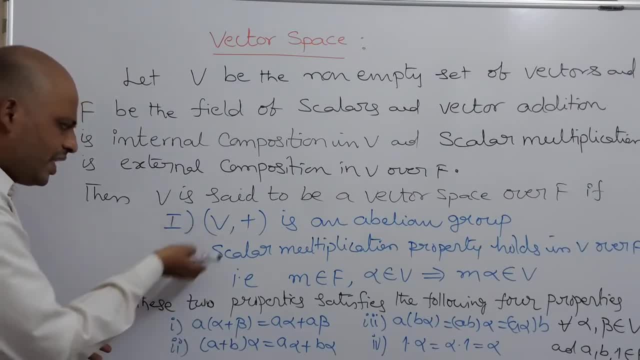 These two are known as major conditions. These two conditions together satisfies the following four properties. The first one: a into alpha plus beta is equal to a alpha plus a beta. Second one: a plus b into alpha is equal to a alpha plus b alpha. 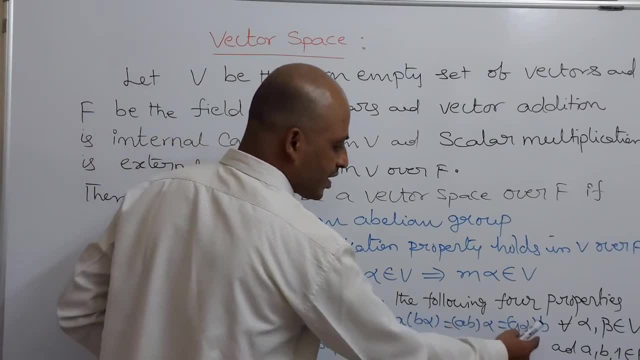 Third one: a into b- alpha is equal to ab. into alpha is equal to a alpha into b. Fourth one: 1 into a alpha is equal to a alpha into b. Fifth one: a into alpha is equal to a. alpha into 1 is equal to alpha. 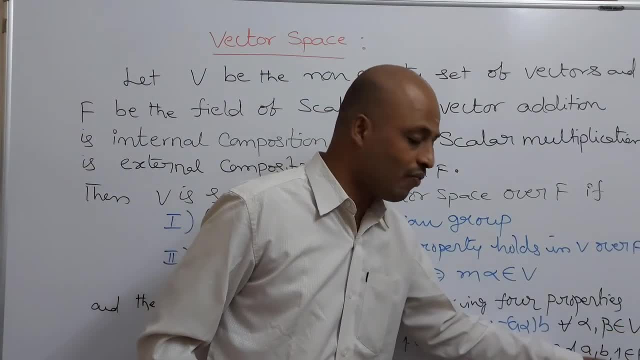 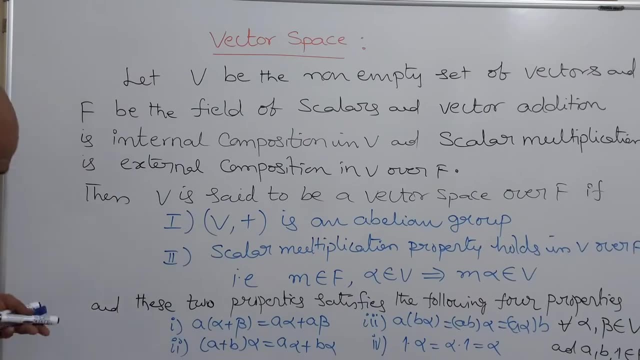 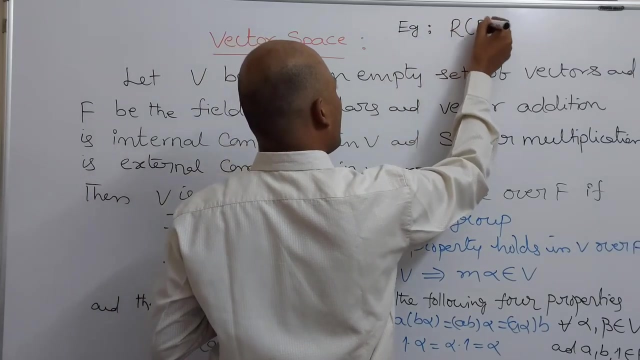 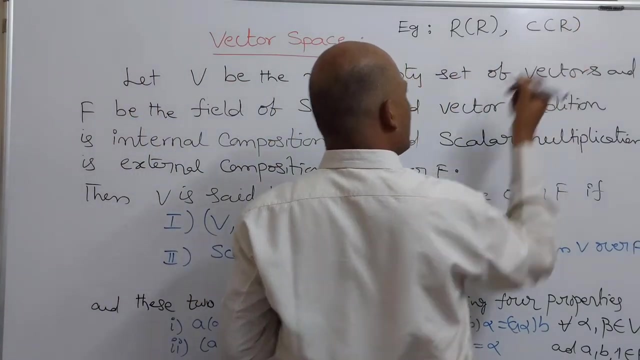 For all. alpha beta belongs to V. a comma, b comma 1 belongs to the field capital F. Yes, this is the definition of vector space. You can see the more examples for vector space. The following are simple examples for vector space: R of r, where capital R is the real numbers, R of r is a vector space. 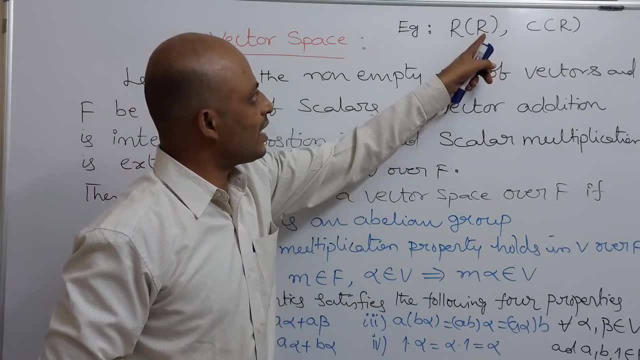 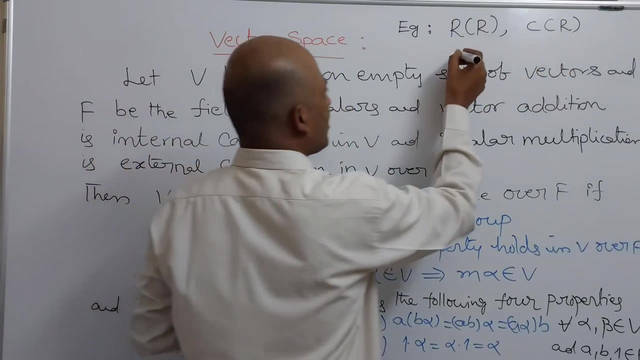 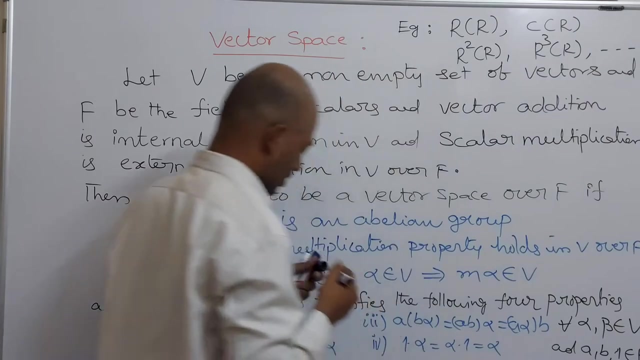 C of r is a vector space. This one represents field, this one represents the set field. set of vectors means V of f And R. square of r is a vector space, R cube of r is a vector space, and so on. These are the very basic examples for the vector space. 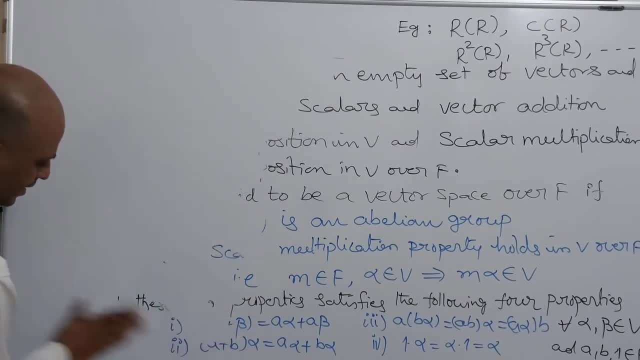 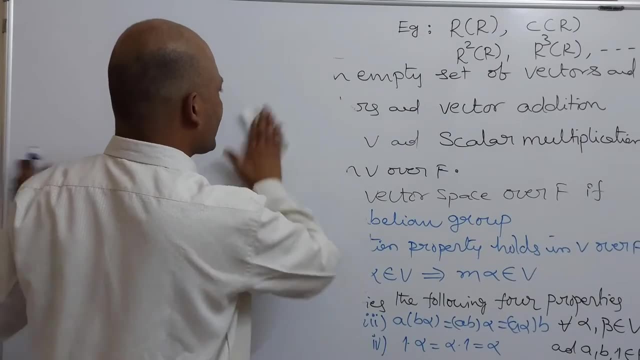 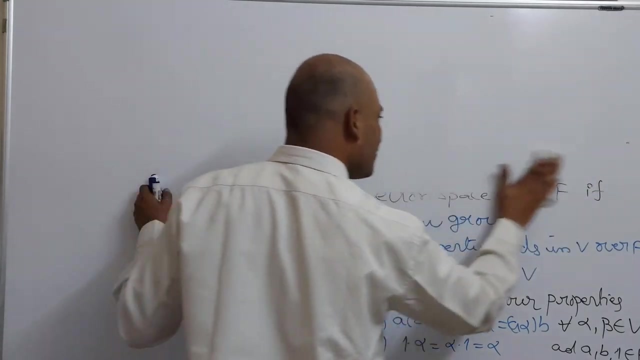 After this definition, let us see one important note point. If the field is the set of real numbers, then the vector space is known as real vector space. If the field is the set of complex numbers, C, then we say that the vector space is a. 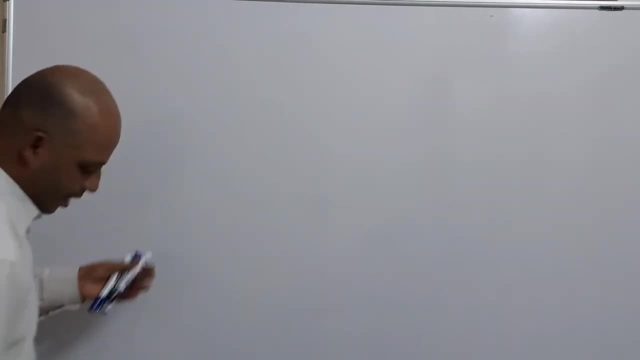 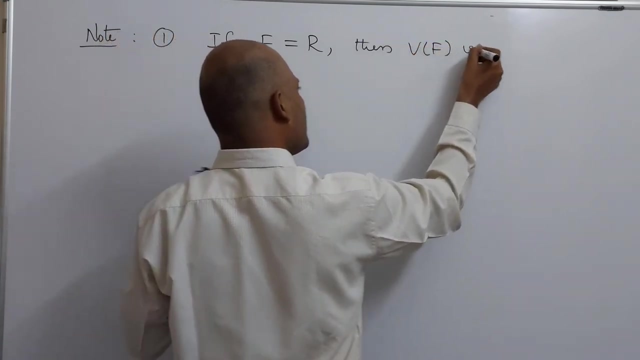 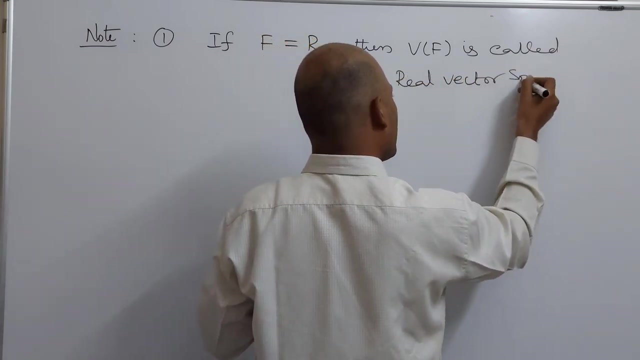 complex vector space, One of the important note point. remember that. let us see that one note point. The first point: if the field capital F is equals to R, Yes, Then V of f is known, as is called or is said to be real vector space, real vector space. 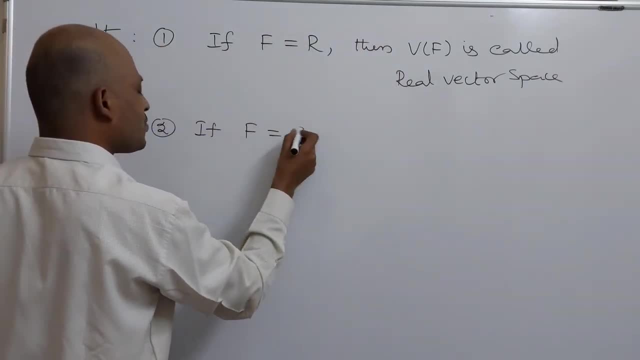 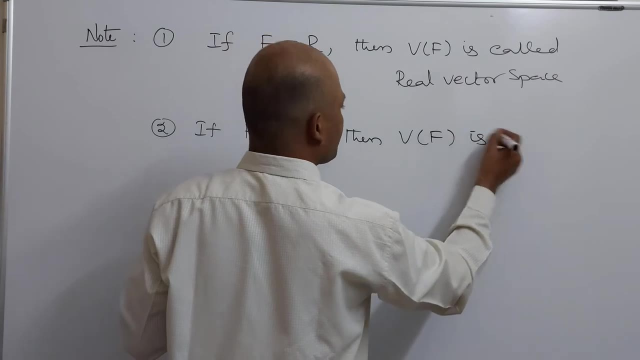 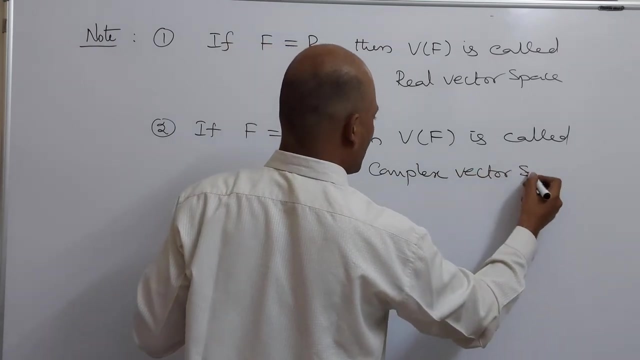 And the second point: if capital F is equals to C means the field is the set of complex numbers. then V of f is called V of f is called complex vector space. complex vector space. Let us see the one more note point, third one: 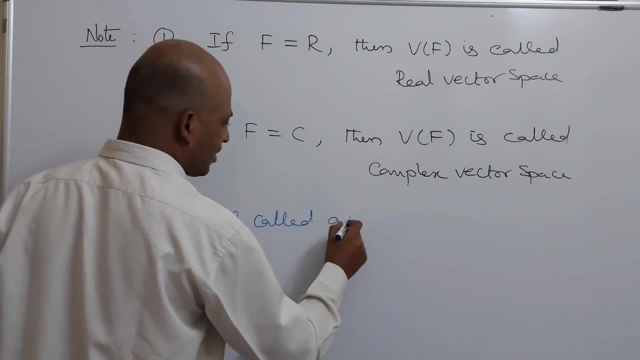 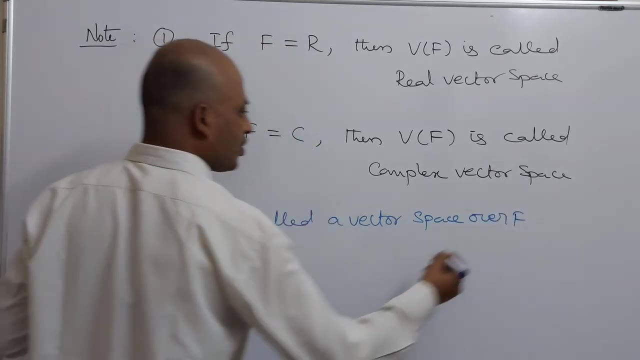 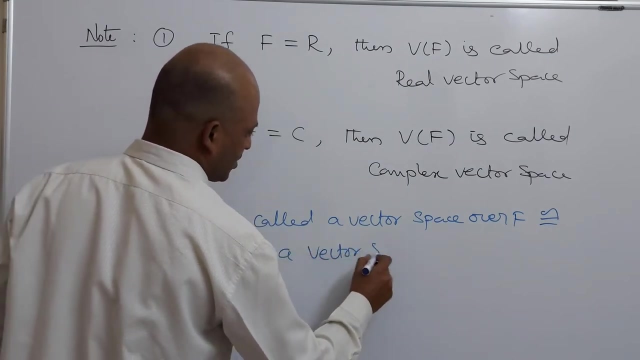 Capital V is called a vector space over capital F, a vector space over capital F. It is also denoted by simply: V of f is a vector space, V of f is a vector space. V of f is a vector space, or in another words, V is a vector space. 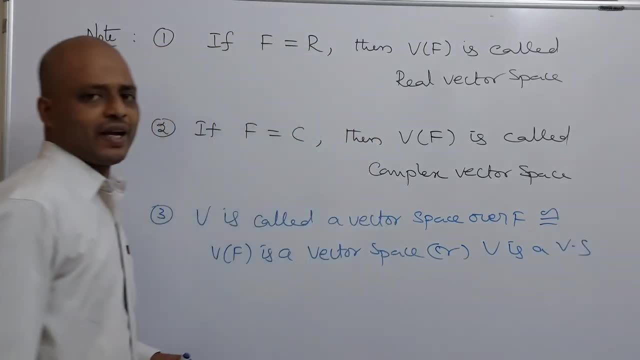 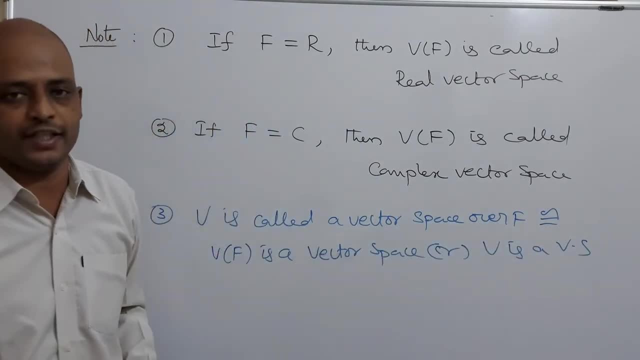 space, or simply V is a vector space. You assume that F is the field, F is the field And in general, in general, R of f, R of r means. this term represents field, this term represents V, R, square of r. this term represents F, this term represents V. So V of f is equal. 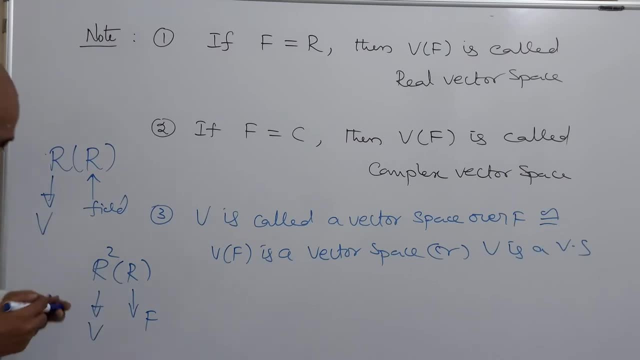 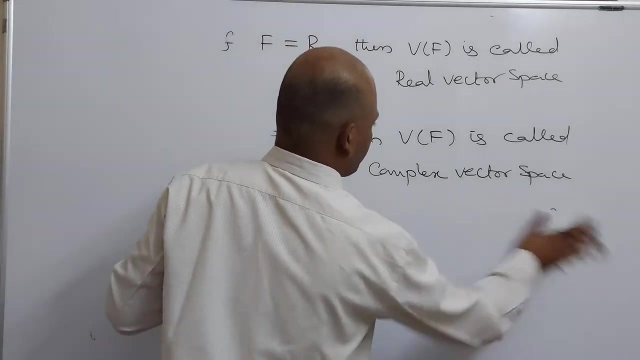 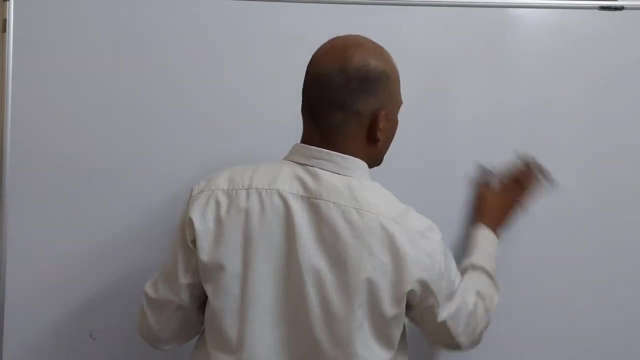 to V. This term represents V. Observe that These are the basic examples and simple points to remember about the vector space. Now let us see. next. let us see the vector subspace definition. Before going to see the vector subspace definition, we learn one simple definition which is known. 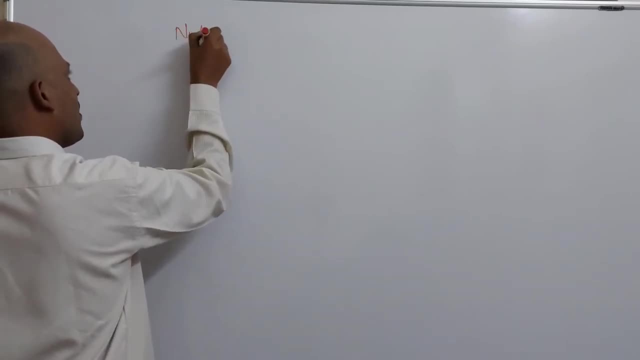 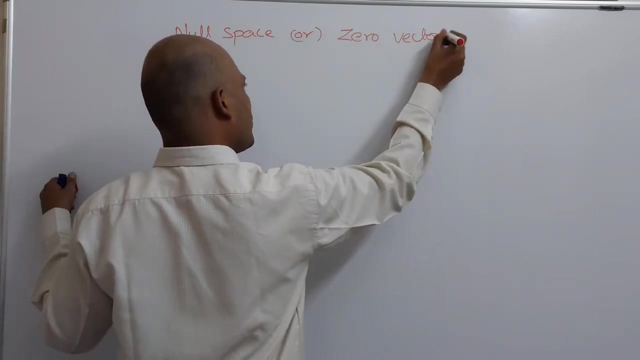 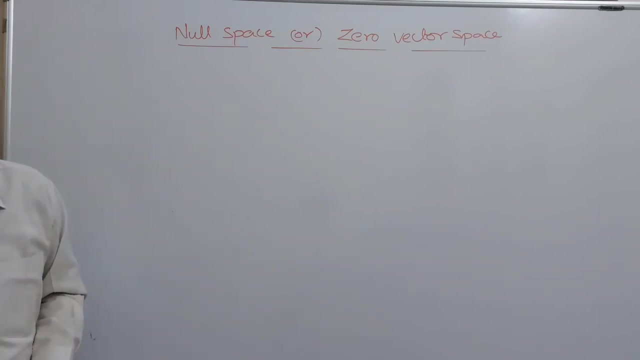 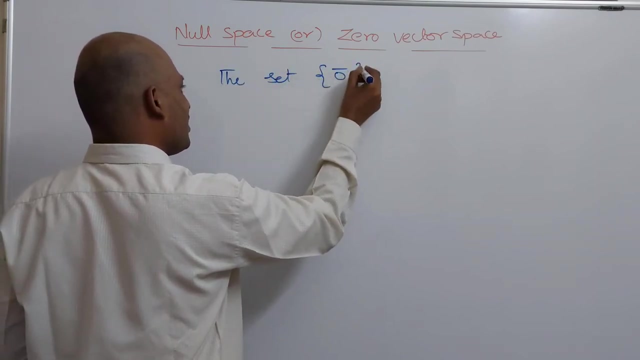 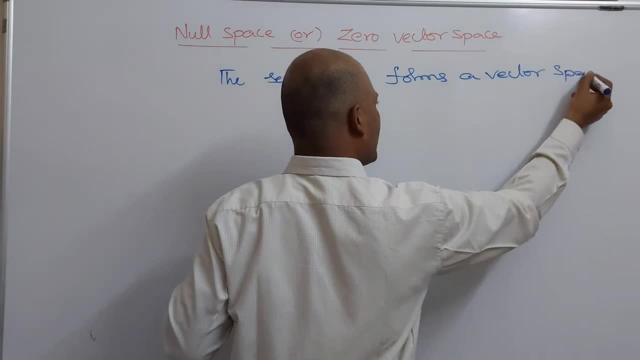 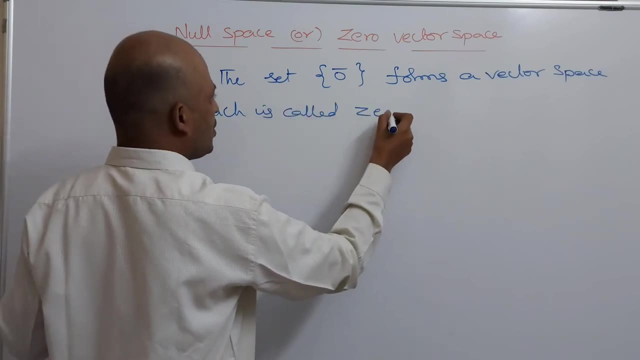 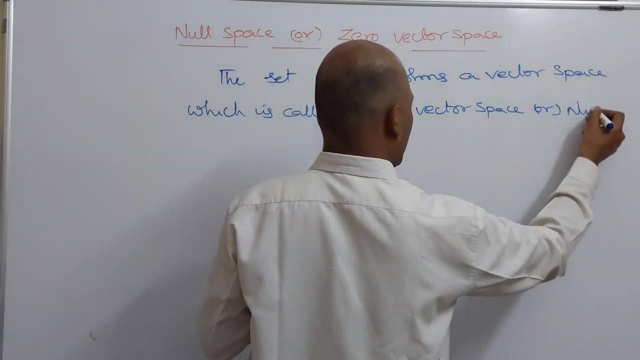 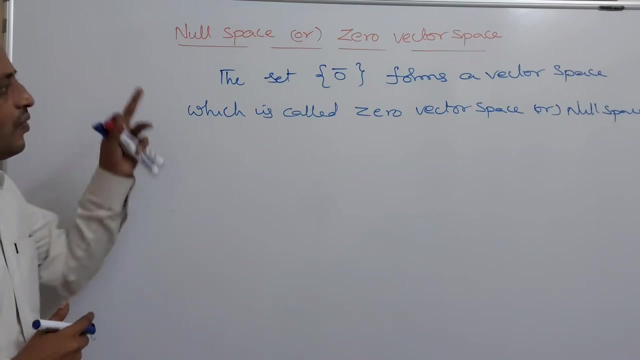 space. a vector space forms a vector space which is known as or which is called, which is called zero vector space, zero vector space or null space. null space, The set having only zero vector. the set having only zero vector forms a vector space which: 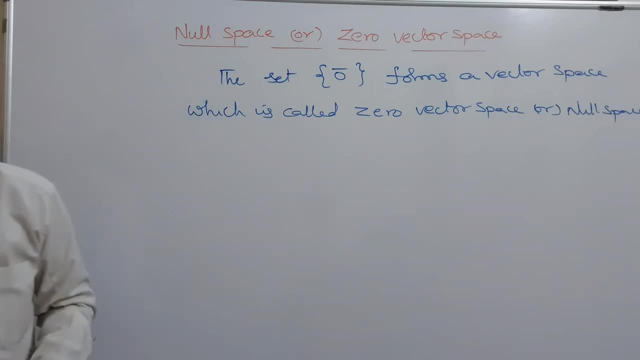 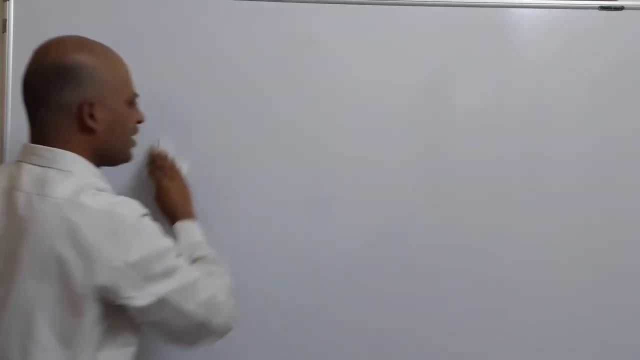 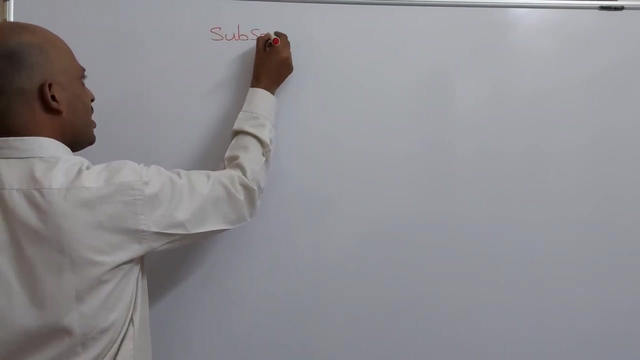 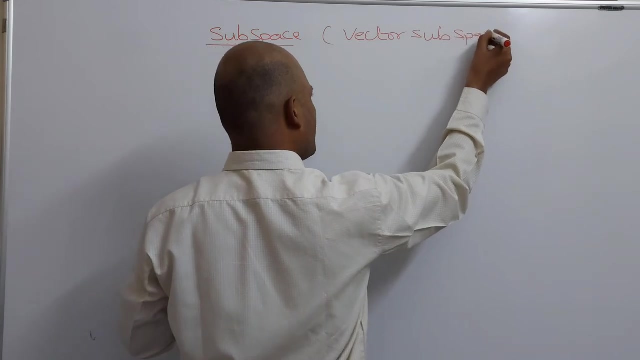 is called the zero vector space or null vector space. Null vector space. Null vector space, No vector space or null space. simply. Now let us see the definition of subspace, one of the very, very important definitions: Subspace, which is also known as vector subspace, vector subspace. 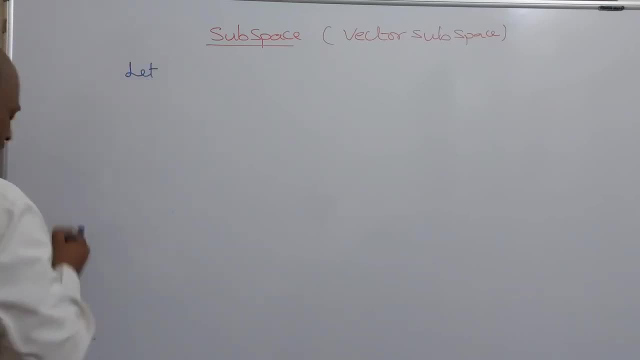 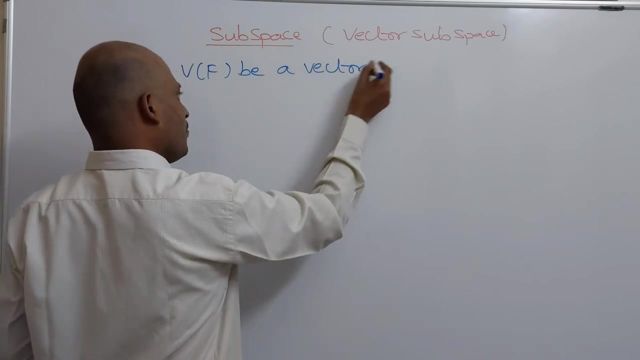 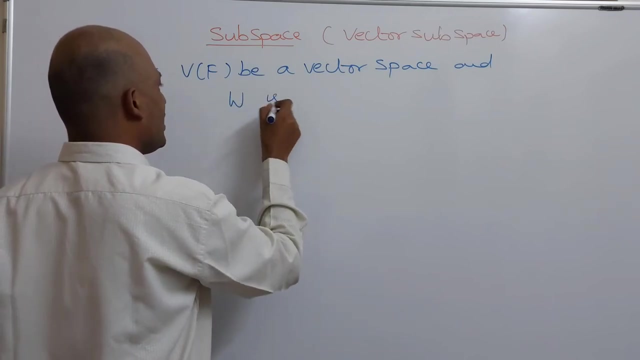 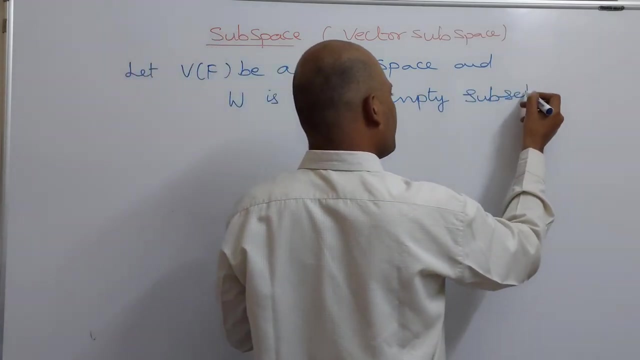 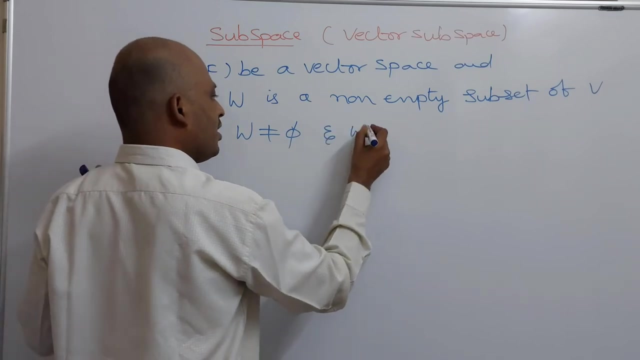 Let V Be a vector space. Let V of F be a vector space, V of F be a vector space, And W is a non-empty subset of V. W is a non-empty subset of V, That is, W not equals to pi And W is subset to V. 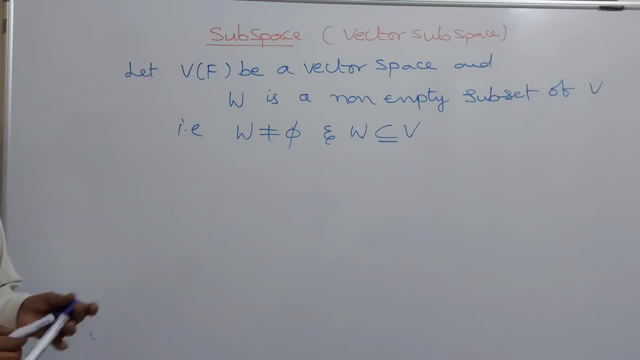 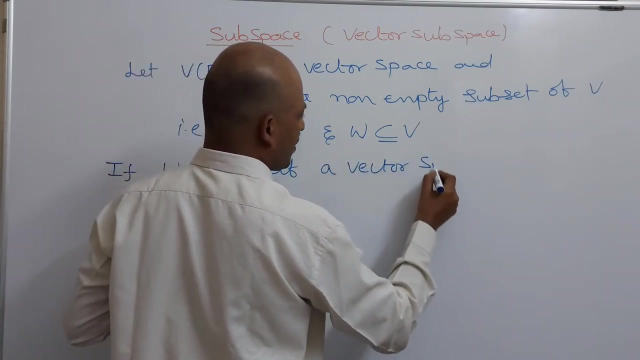 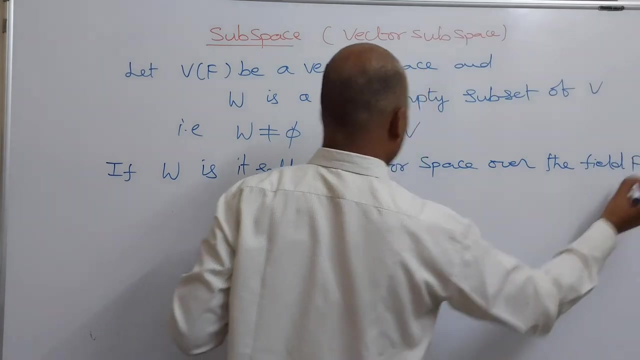 Subsets are equivalent to V. You can write any one: W is subset to V or W is subset are equivalent to V. If W is itself a vector space, If W is itself a vector space Over the field capital F. Over the field capital F.